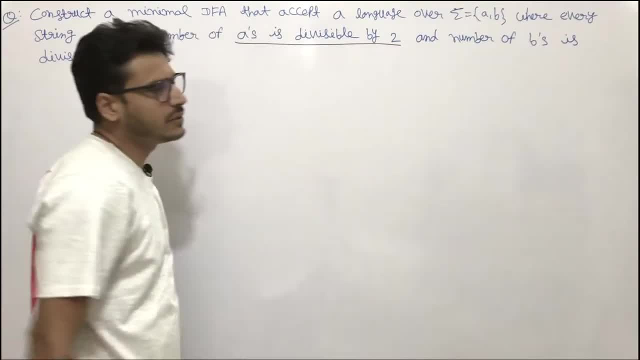 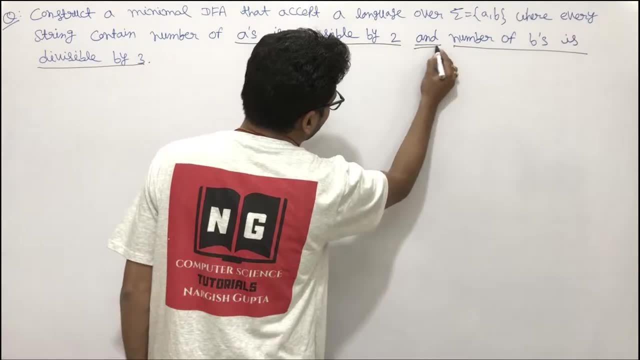 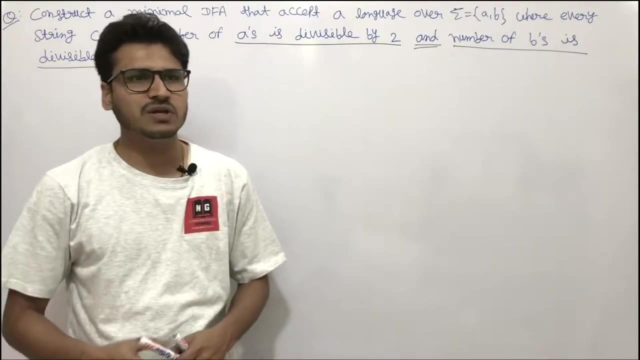 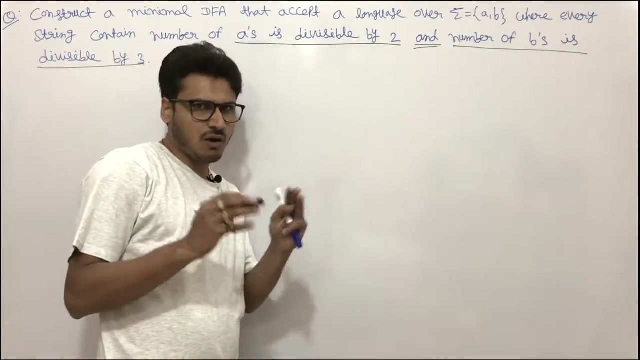 number of A's is divisible by 2 and number of B is divisible by 3.. Remember, and operator is here Means in this question I am constructing a different type of DFA. In previous videos we had constructed a simple DFA. Now here is compound. DFA means there is a combination. 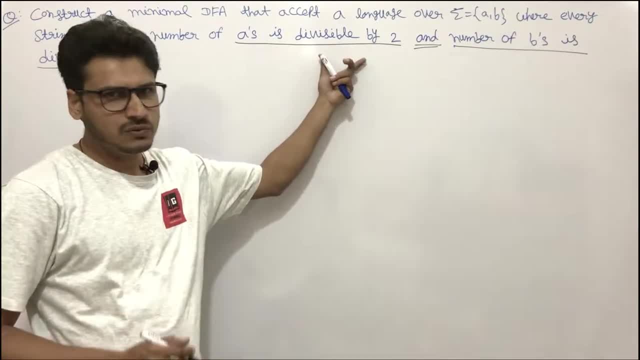 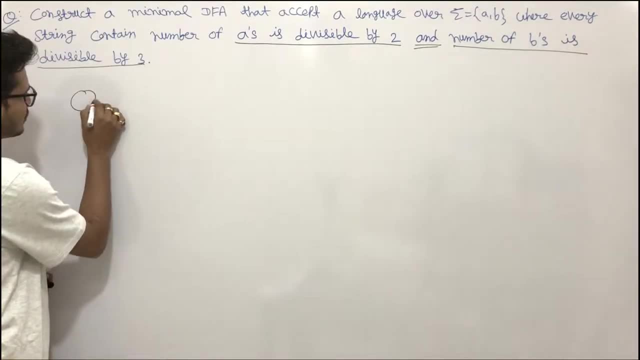 of two DFA's here. I have one DFA divisible by 2.. The other DFA is divisible by 2 and I have one DFA divisible by 3.. So first of all, we construct a simple DFA for divisible by 2.. So, as we had constructed, I have constructed a DFA for divisible by 2.. A is divisible by: 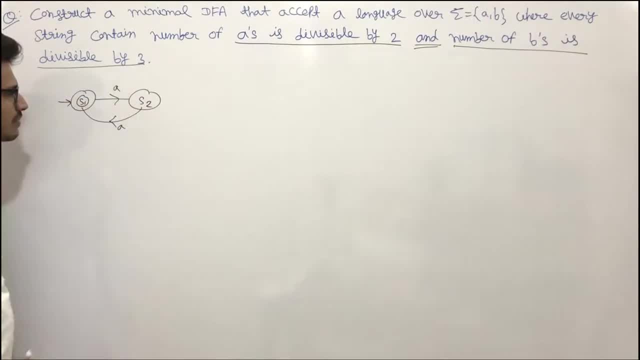 2. S1 is a starting state and S1 is my final state And A is divisible by A, So any combination of B can be there because we have A and B given as input. So this is my DFA 1.. So 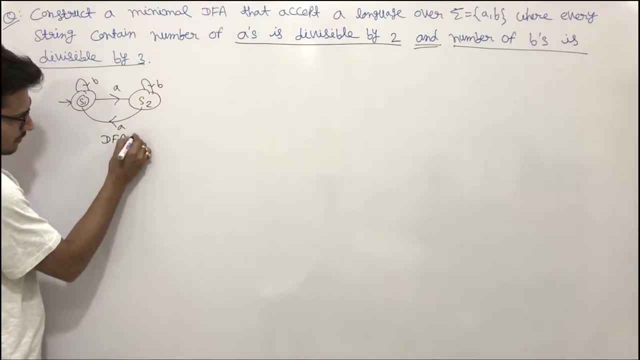 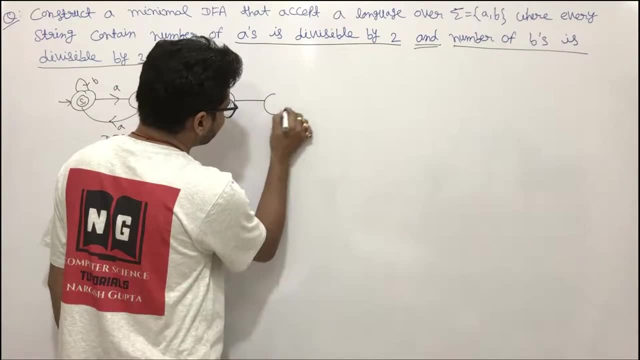 I can say this: This is my DFA. 1. This is my divisible by 2.. Now let's make it divisible by 3. Means divisible by 3.. What is divisible by 3?? B is my 3 divides 1 B, 2 B and 3 B. Take from: 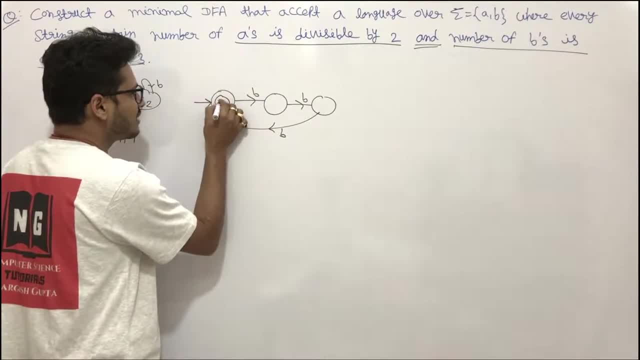 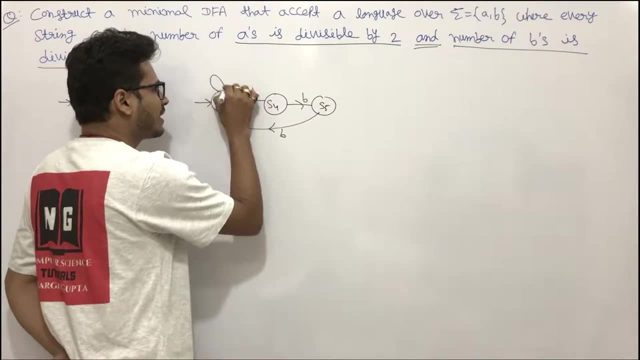 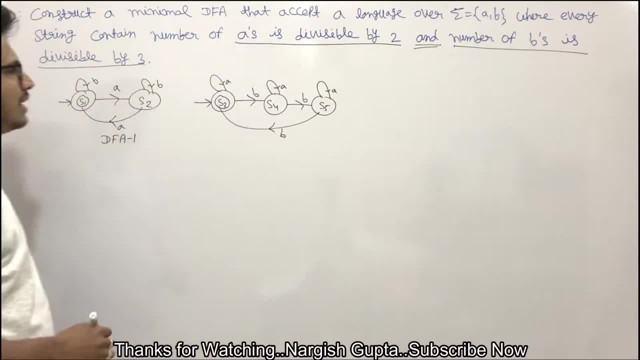 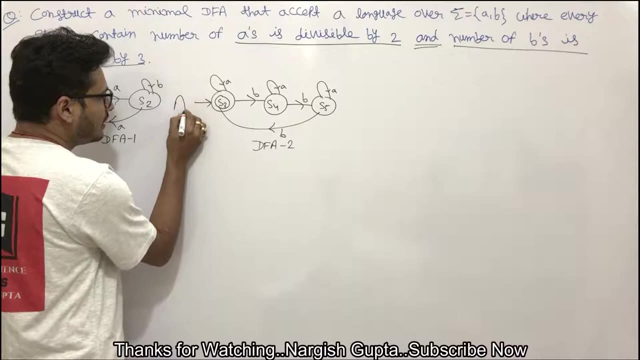 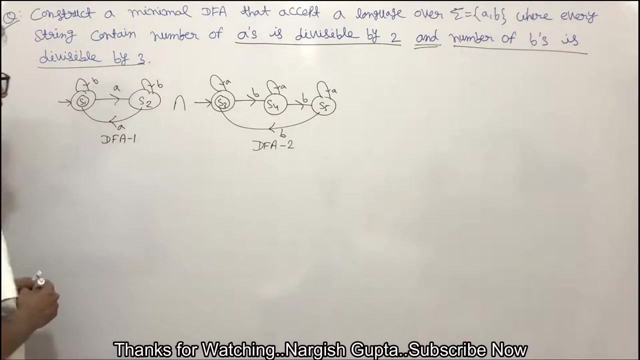 A can be there, any number of A can be there. So this is my DFA 2, which is divided by B, which is divided by 3.. Now, in both these DFA's, we have to perform intersection and end operator. Now, to perform end operator, we have to do some simple rules. So first, 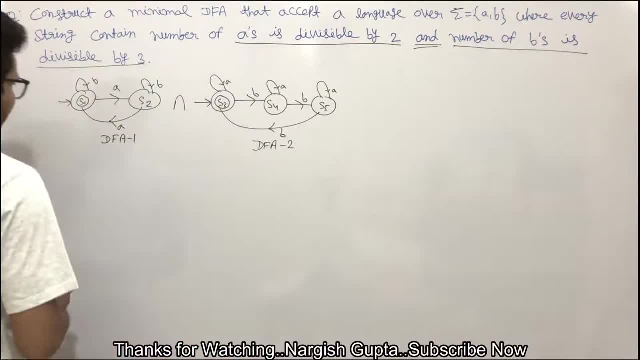 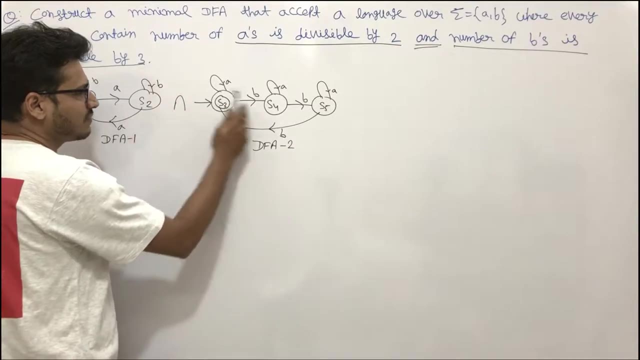 rule is that What we do, What we have to do, What do we have to do? the cross production that you are doing here is: multiply S1 by S3, multiply S1 by S4, multiply S1 by S5, multiply S2 by S3. 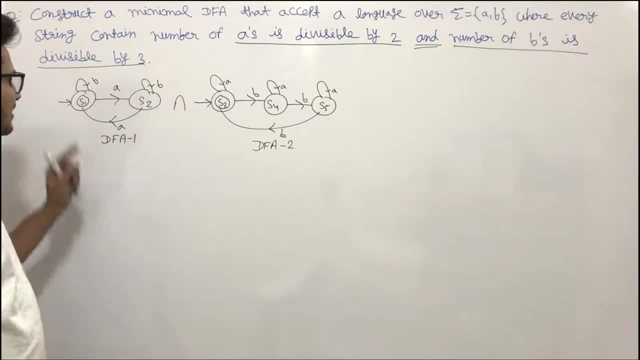 multiply S4 by S5. so if we talk about total states, so 2 cross 3. so if I talk about 2 cross 3, then how much is being made here? total 6 states. so first I will make such a DFA in which DFA I have. 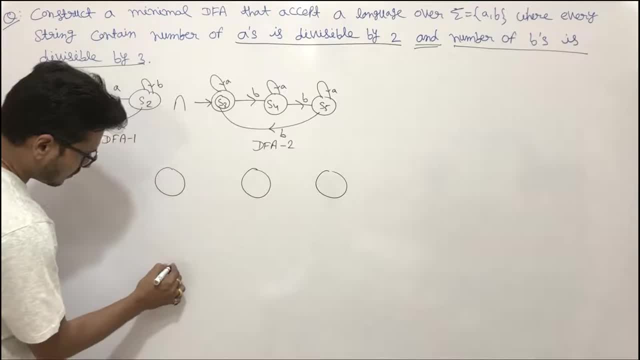 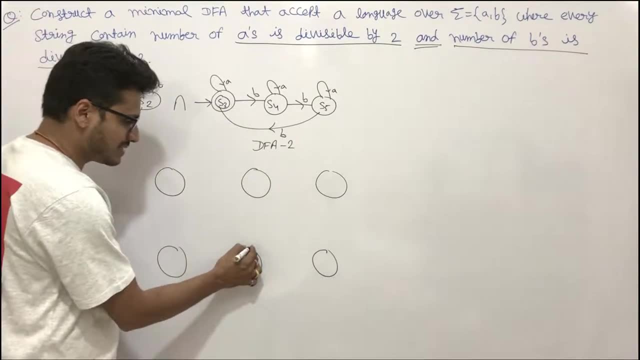 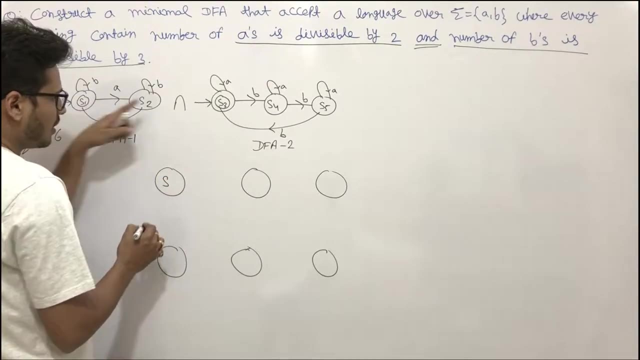 1,2,3,4,5 and 6 states. so this is my total number of states. now what I have to do, because I am doing cross production, this is my state S1. cross production of this is done by S3, so S13 is my first state. 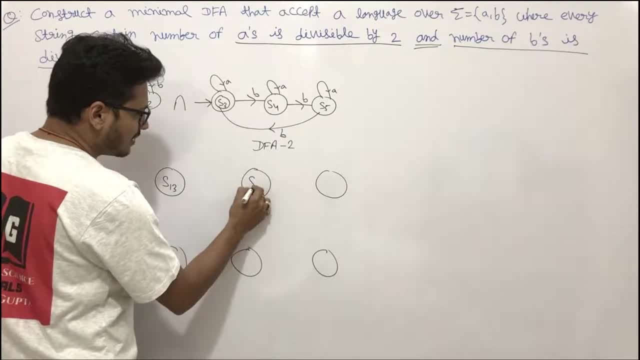 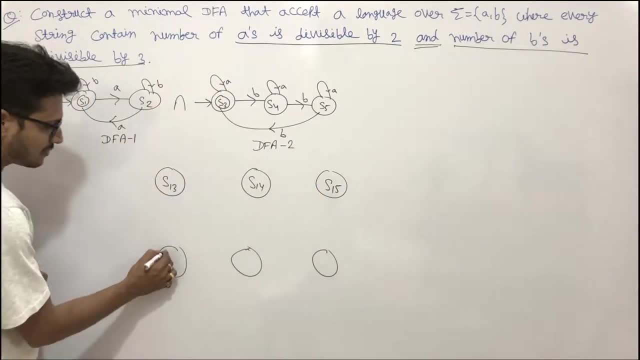 cross production of S1 is done by S4, so S14 is done. S15 is done by S1. S2 is done by S3, so S23 is done. S24 is done, S25 is done. so these are my states. rule number next is: 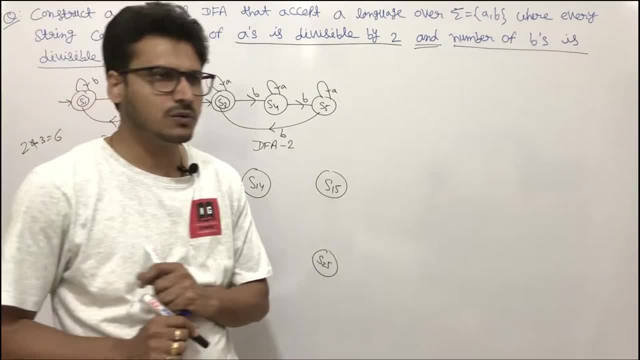 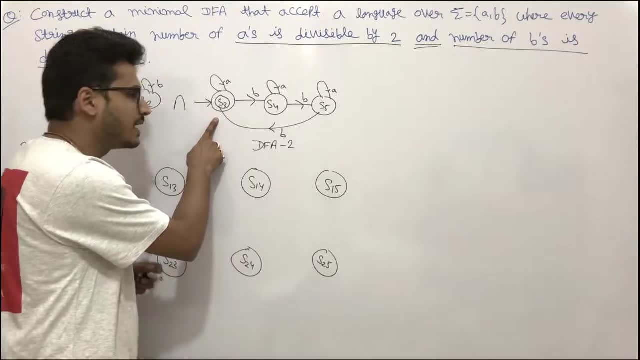 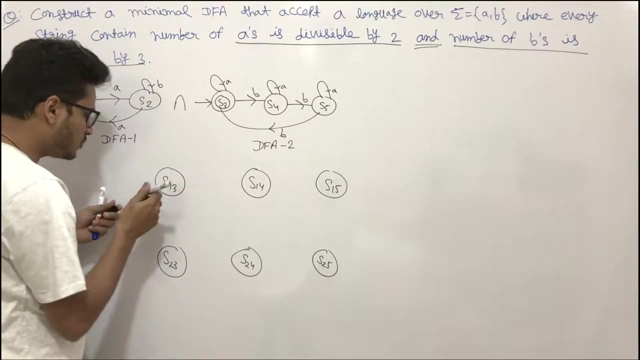 whatever are our final states, make them final states. now, if you will see here, S1 is my final state. if you will see here, S3 is my final state. means whatever production we have done- cross production- S13 is done, so S13 is my state. that will be my final state. 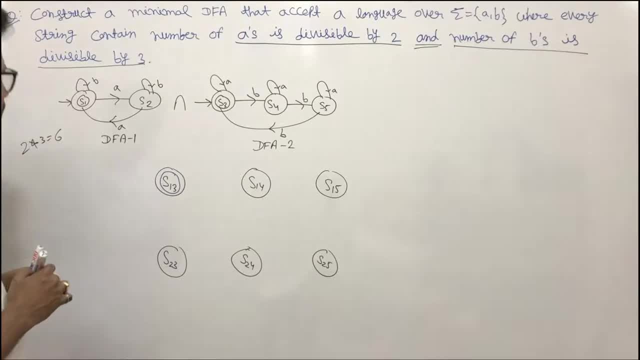 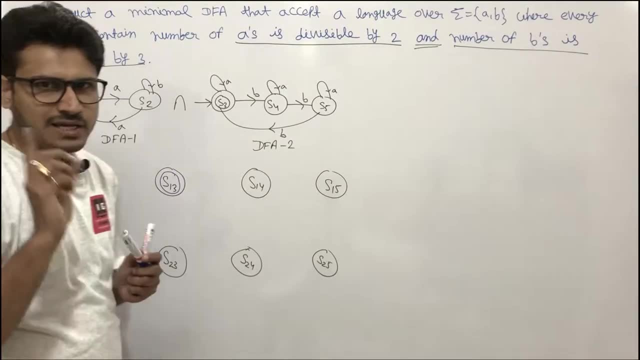 so what we have done with S13, we have made it final after that because, see, S13 is not there. this is my state after that: whatever initial- because initial can be one state- final can be multiple. now, in initial state, S1 was initial and S3 was initial. 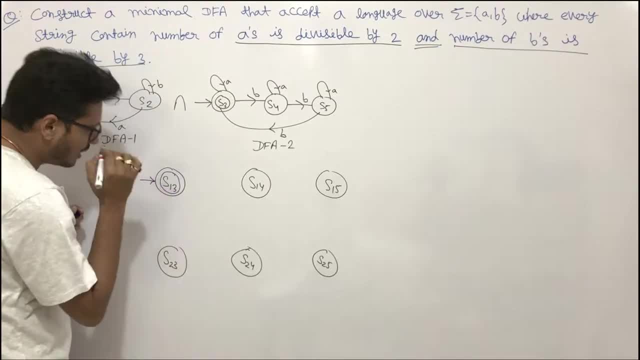 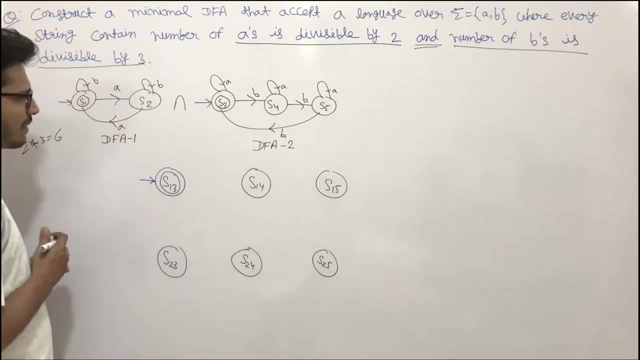 so what will be my state? S1 and 3 will be my initial state. so this is my final and initial state. now it is simple: we have to do transaction where transaction is happening. we will do transaction there. how see S1, S1 with B transaction. 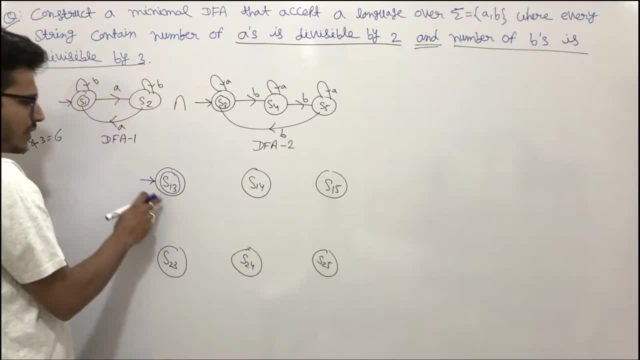 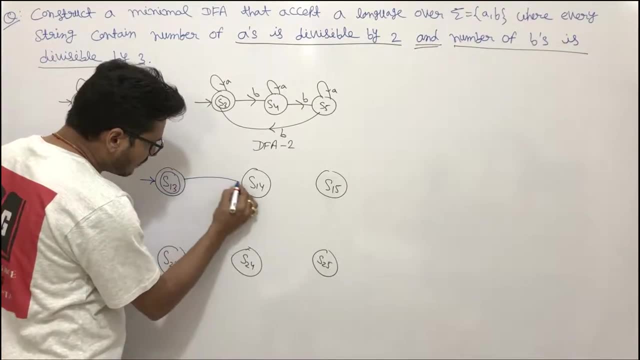 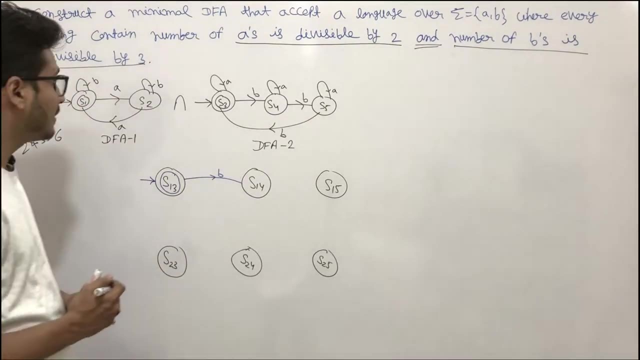 where are you going? you are going to S1, so S1 with B transaction. you are going to S1, so from here with B transaction. can I go to 1?? yes, I can go to 1, there is no issue then after that. now see this: 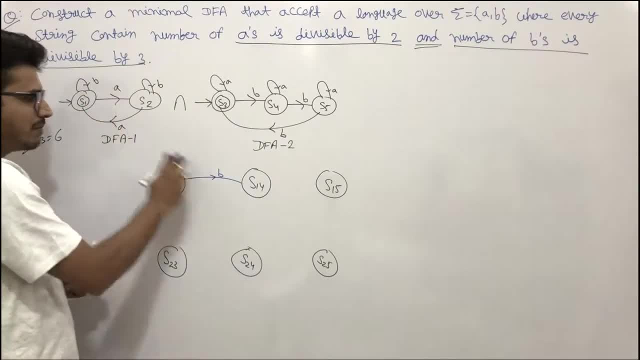 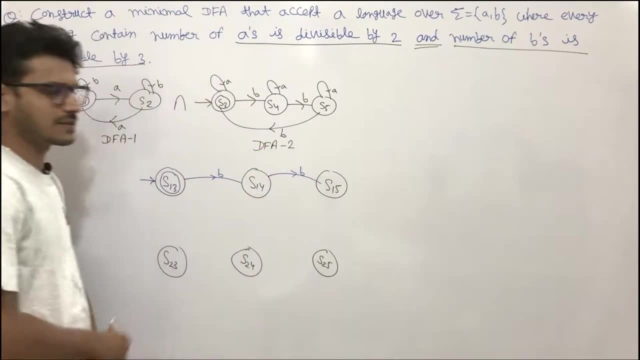 where are we going with S1 with transaction B to S1? but if I see here S1 with B again going to S1, so here also I can do transaction of B, after that from S1 to A. where are you going to S2? state. 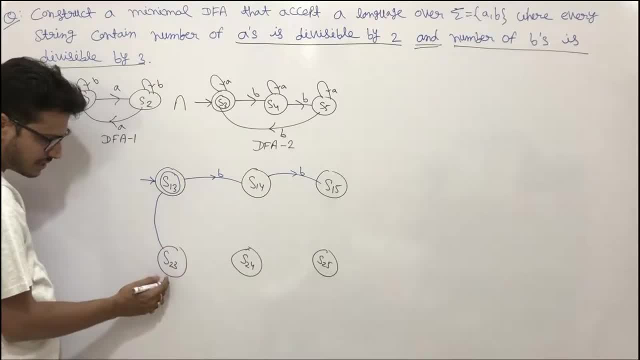 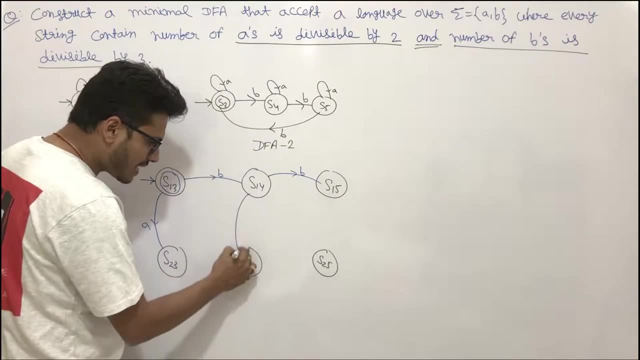 so from S1 to A, you are going to S2. state, so 1 S2 is your. this, and see, this is also your S1. from S1 to A. where are you going to S2? so from A, you are going to S2. 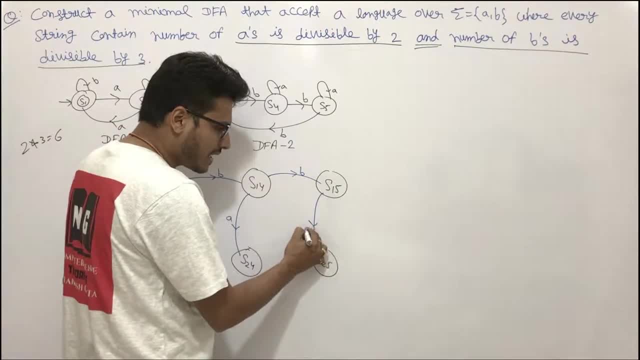 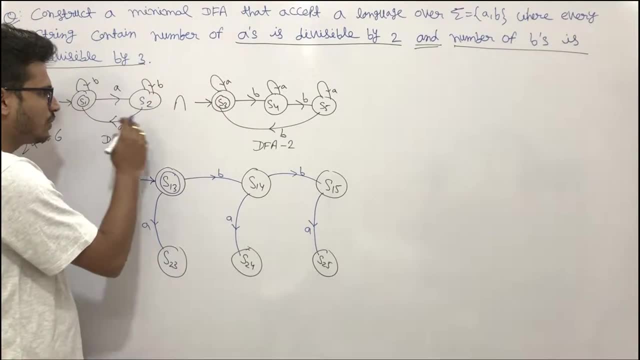 this is also my S1, so from S1 to A, where are you going to S2? so we are going to S2 then after that transaction of S1 is completed. now we are coming to S2 as soon as we come to S2. 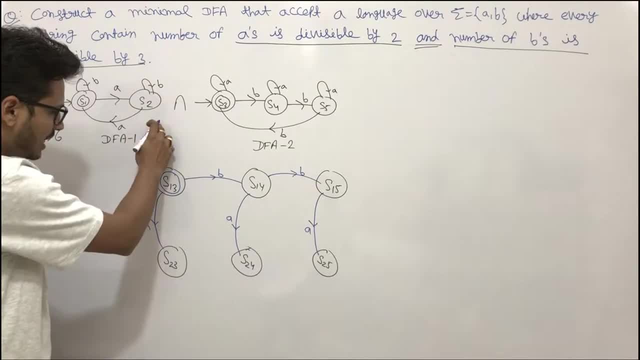 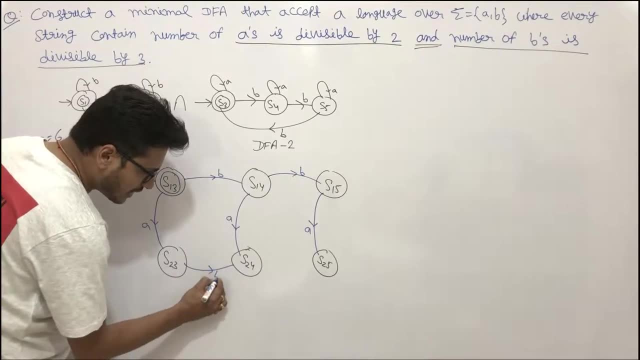 you see, from S2 to B, we are going to S2, S2 to B by taking transaction. we are going to S2. I took a transaction from S2 to B and went to S2. but if you want to go from S2 to B and go to S2, 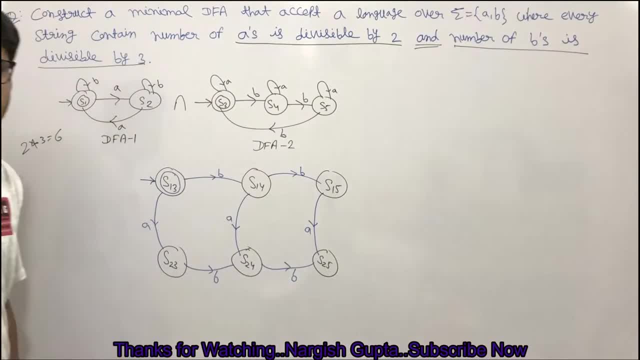 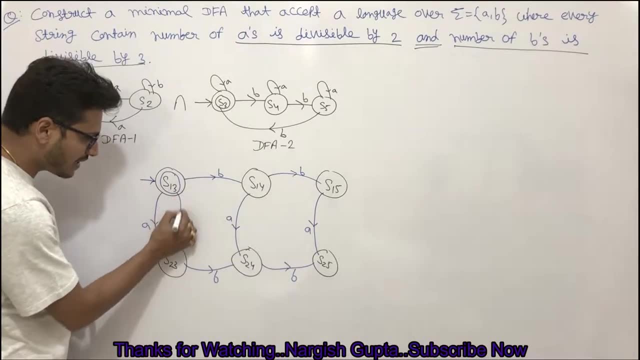 then the same situation is here. so I took a transaction from B and went to S1. after that, from S2 to A, you are coming to S1, so this is my S2 by taking A's transaction. where did I come to S1? 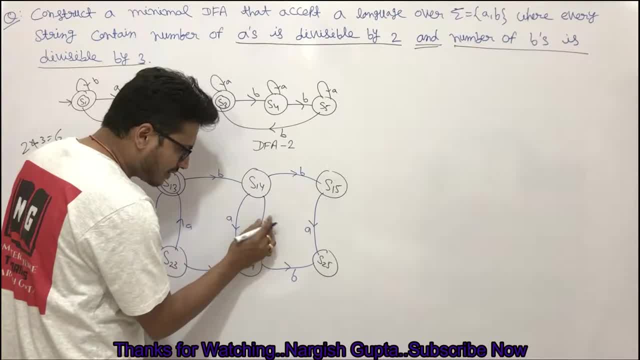 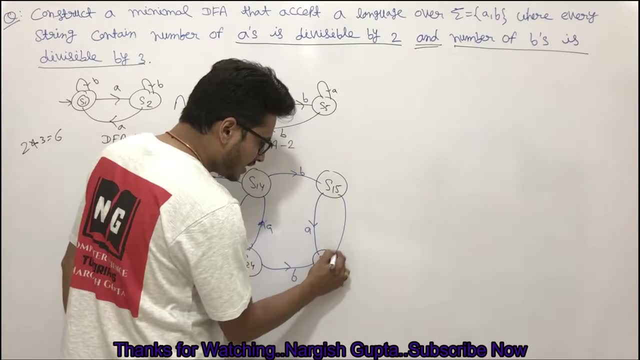 this is also my S2 and this is S1. so by taking A's transaction, where did I go? by taking A's transaction, I went to S1. this is also S2 and this is S1. so by taking A's transaction, I went to S1. 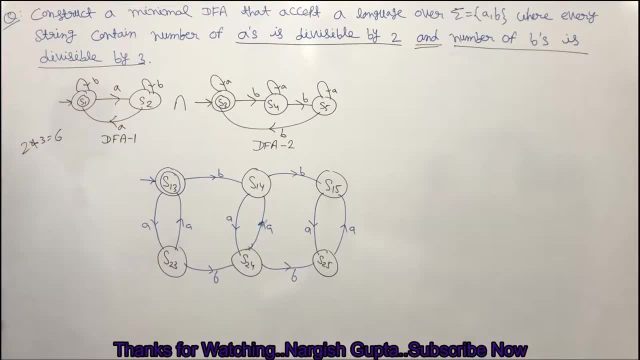 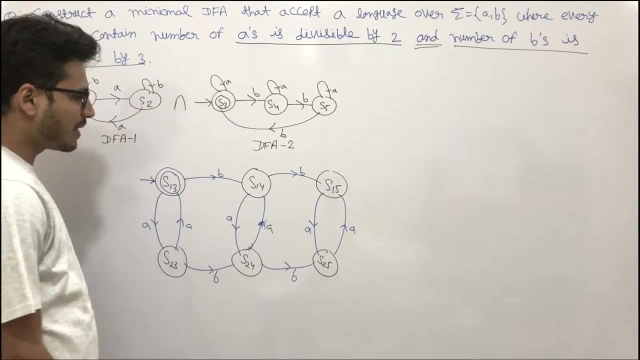 now, this much is complete means DFA1's task is complete. now let's come to DFA2. in DFA2, you see, by taking A's transaction from S3, where are you going? by taking A's transaction from S3, you are going to S3. 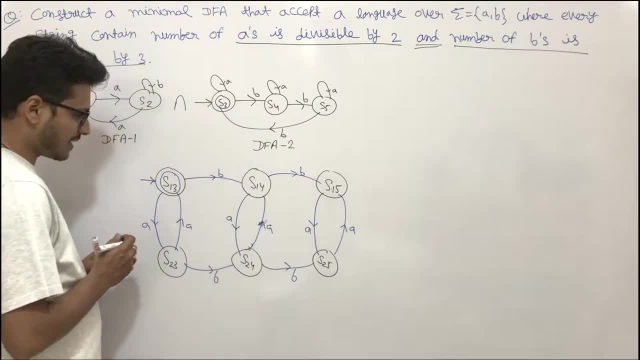 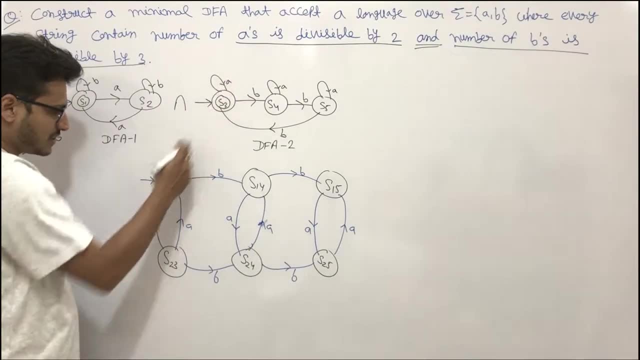 so now let's see where is our S3?. this is S3 and this is S3. is there any other S3?? then, by taking A's transaction from S3, where are you going on? S3 B: taking A's transaction from S3. 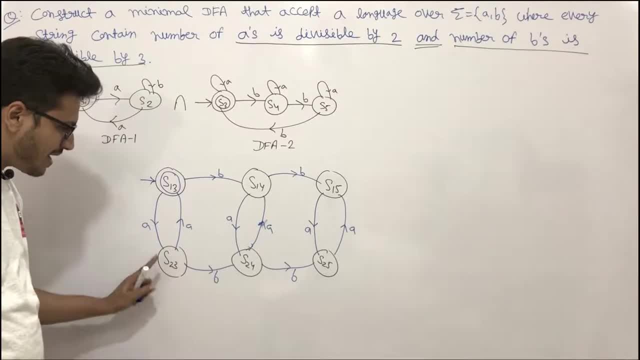 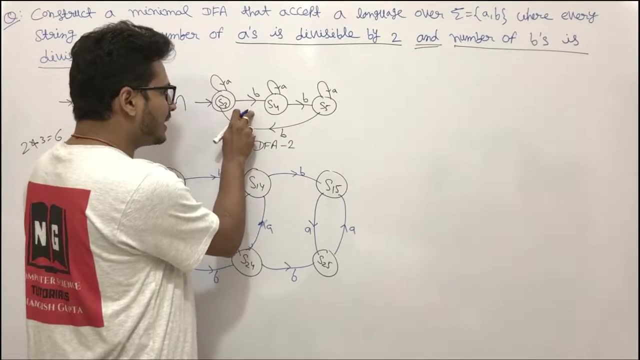 where are you going on S3? this means that from that state to that state and from this state to this state, by taking A's transaction, we have already done it. Next, by taking S3 from B's transaction, you are going on S4. where is your S3? here? 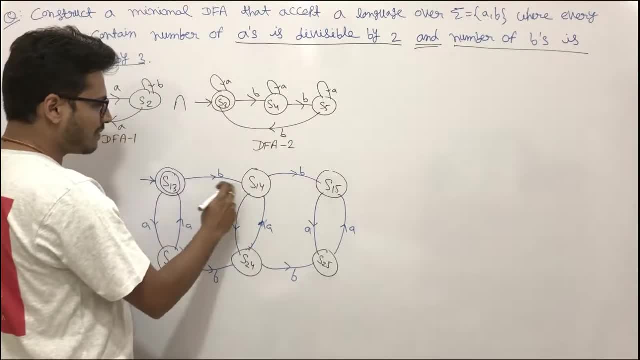 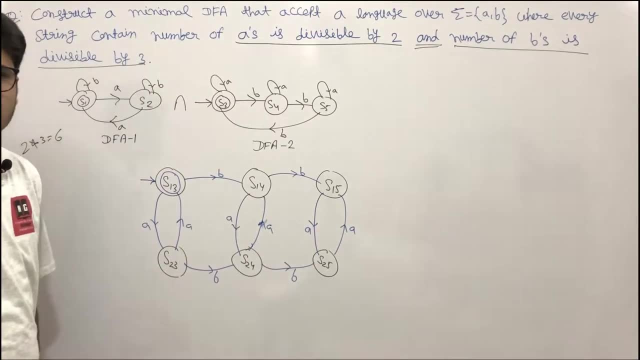 and it is here also, and by taking B's transaction from S3, you are going on S4. this one is B Free from S3, from B to S4, from S3 to B to S4, we have done this work also. now we come to S4, now. 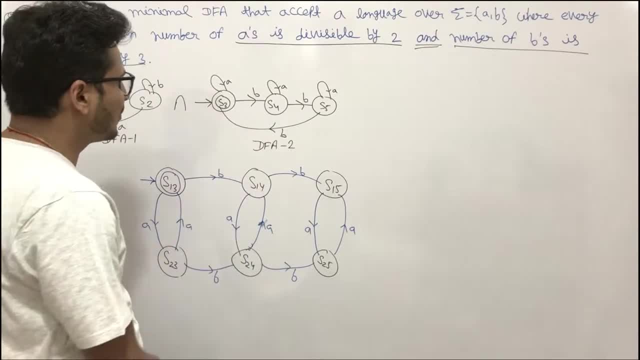 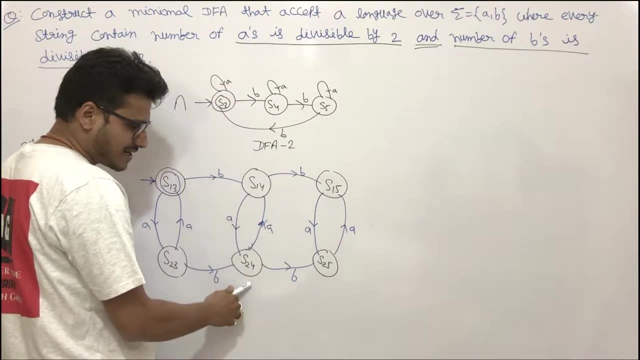 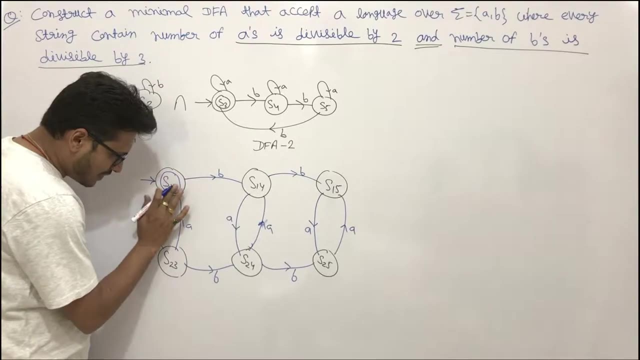 transaction of S3 is done. A and B come to S4, from S4 to A transaction, I am coming to S4, from S4 to A transaction, I am coming to S4,. if you see this individually, this is S1, and if you hide this 1, then this is S3, if you hide this 1, then this is S4, if you. 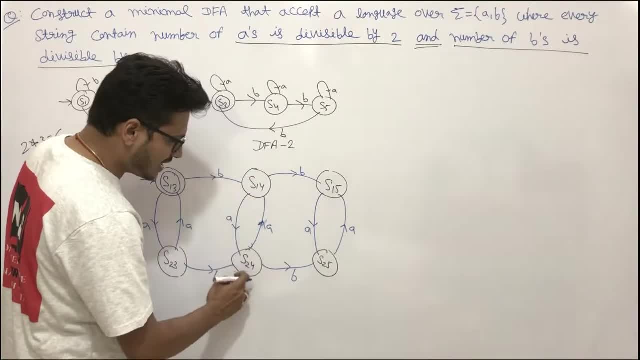 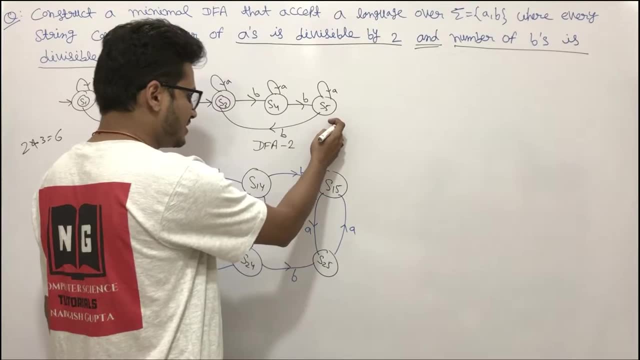 hide this 2, then this is S4, from S4 to A transaction, I am coming to S4, from S4 to A transaction, I am coming to S4, then from S4 to B transaction, I am coming to S5, from. 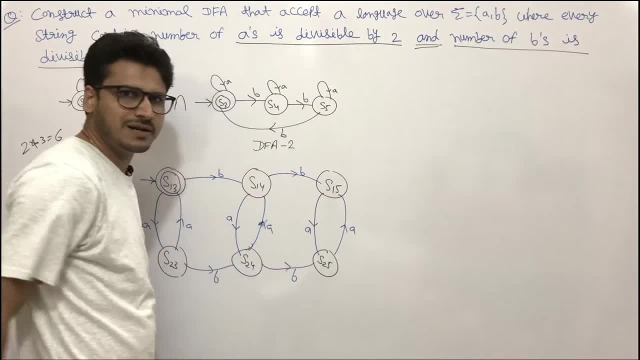 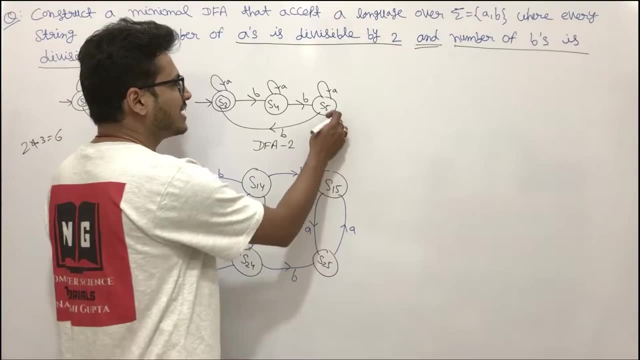 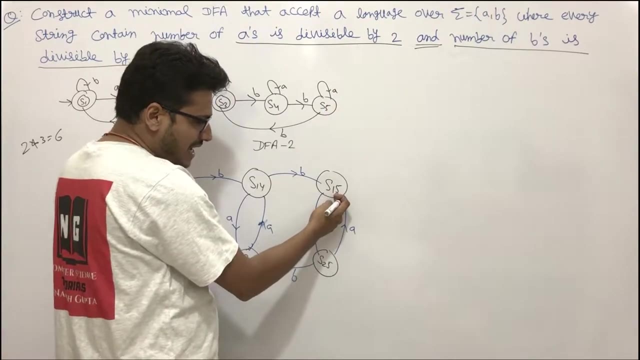 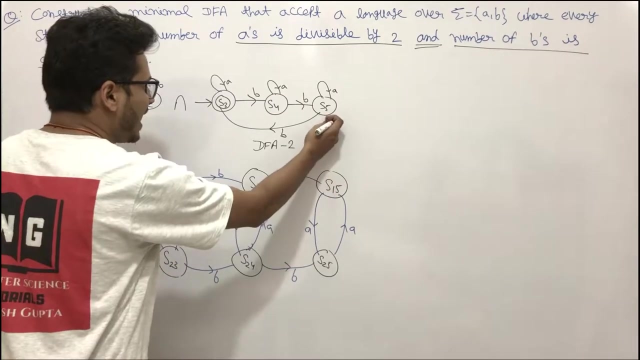 S4 to B transaction, I am coming to S5, and, if you see, from S4 to B transaction, I am coming to S5,. this transaction of S4 is complete. from S5 to B transaction, I am coming to S5, and move from a, from s5 to s5, from a, from s5 to a, from s5, from a to s5 to s5. 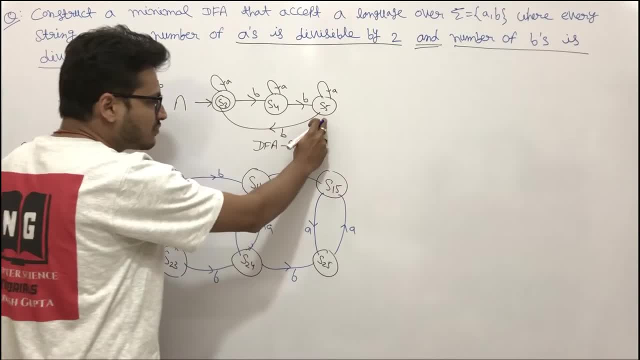 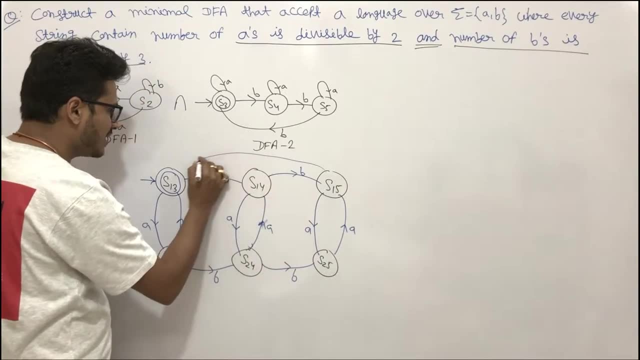 transaction lekar aap s3 par ja rahe hain. s5 se b ka transaction lekar aap s3 par ja rahe hain to s5 se b ka transaction lekar aap s3 par ha rahe hain. but hume yaha par nahi rukna. 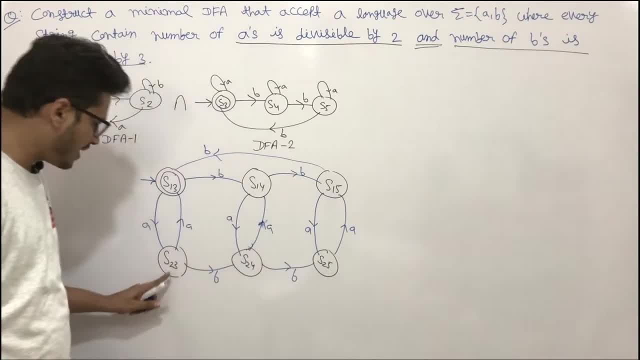 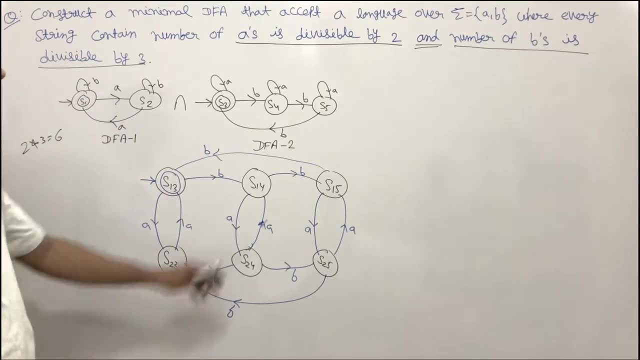 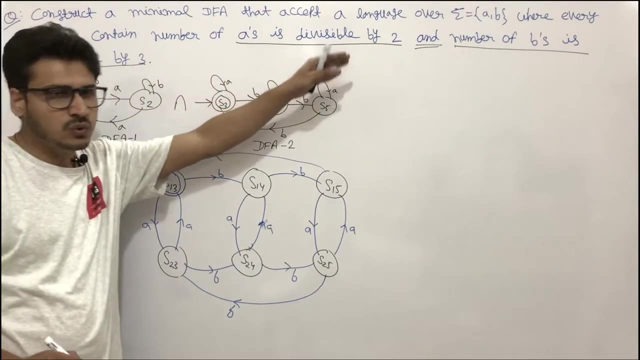 aur b dekhna hai: s5 kaha hai, yaha par s3 kaha hai ek aur yaha par to s5 se b ka transaction lekara. aap kahan pasgThey esi par. Now, this is perfect, complete minimal DFA, which is: a is divisible by 2 and b is divisible.